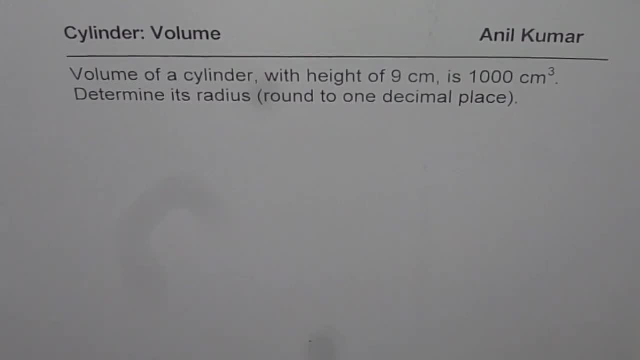 I am Anil Kumar and in this example we will do some backward calculations to find radius of a cylinder. The question here is: volume of a cylinder with height of 9 cm? is 1000 cm cube? Determine its radius round to one decimal place? 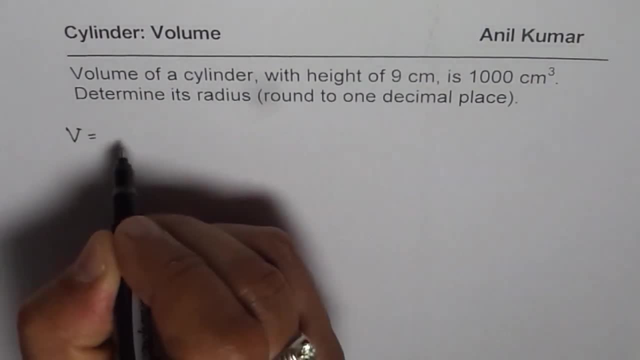 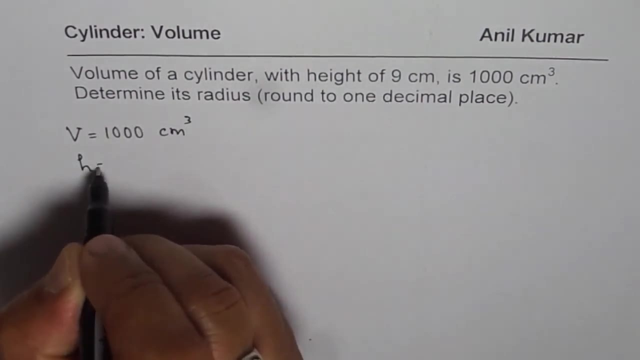 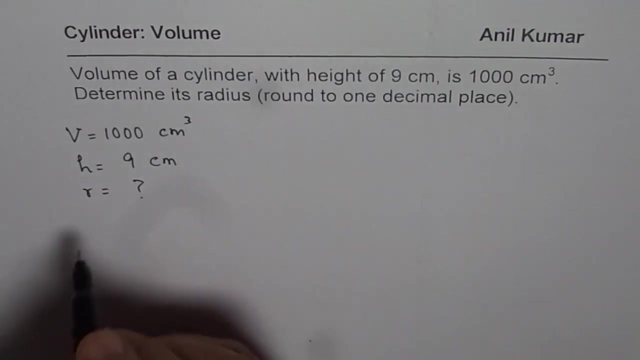 What we are given here is volume, which is 1000 cm cube. We are also given height, which is 9 cm, and radius is something which we need to find. All this is given for a cylinder. Let me sketch one for you. This is a cylinder whose volume is given to us, and this cylinder has height of 9 cm. 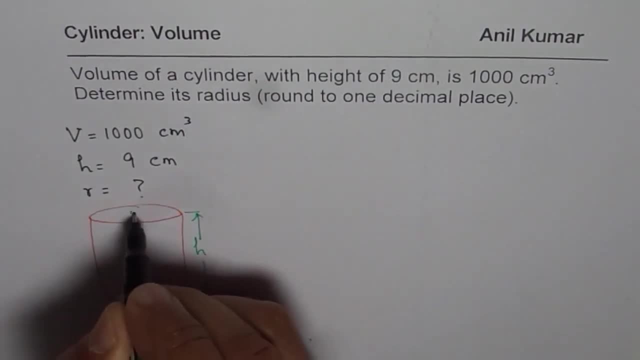 Height of H, radius of R and volume of 1000.. Units are cm. square. Height H is 9 cm. We need to find what radius is. How are you going to find it? Well, you can pause the video, do or solve the question and then look into my solution. 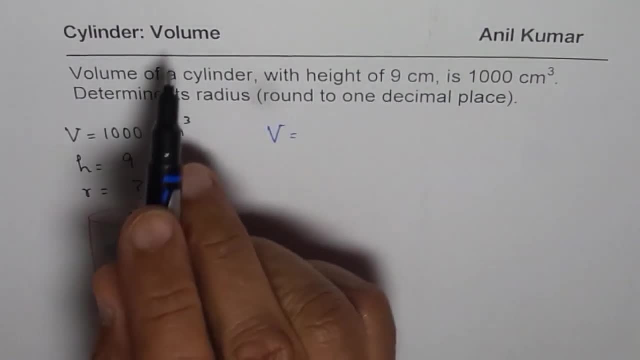 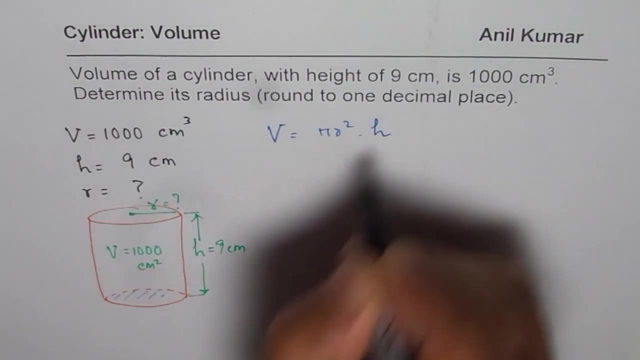 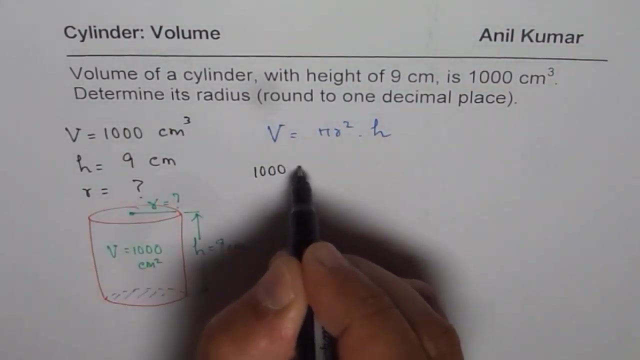 What is the formula for volume of a cylinder Area of the base which is pi, R square times height? That is the formula, And in this formula we are given volume. Let us write down 1000 equals to pi, which you could write as 3.14 times radius. We don't know. 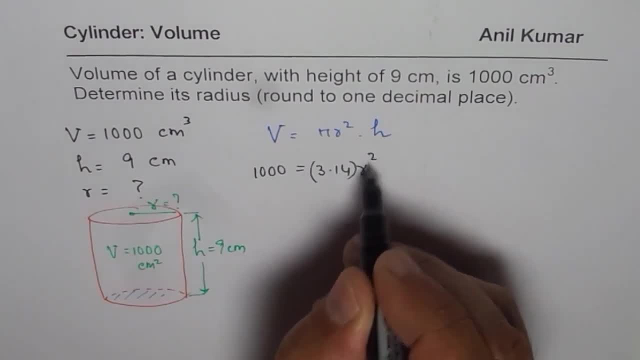 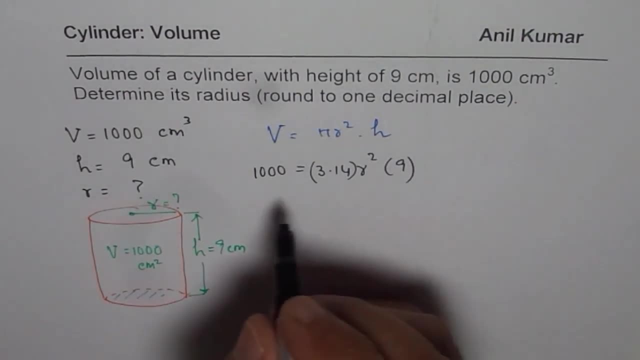 So we will write radius square 3.14 times radius square, and height is 9.. So we can write 9 here. Now you can rearrange the formula So we get radius square equals to 1000 divided by 3.14 times 9.. Right. 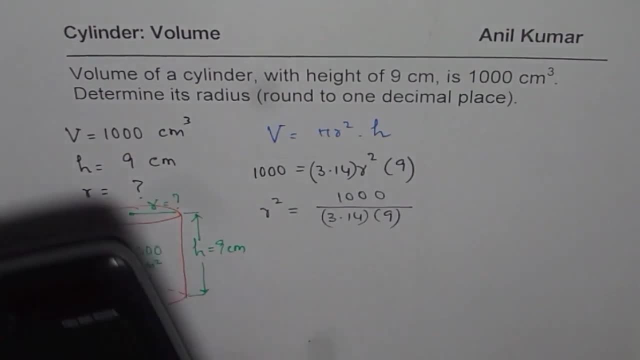 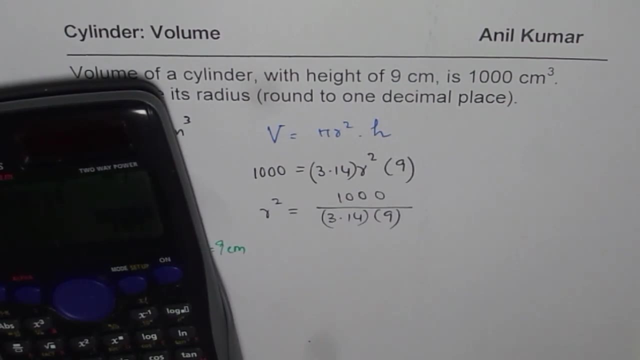 So that is how we can actually find the radius square. So we have 1000 divided by 3.14, and then we can divide by 9.. So we get our answer here for R square as equal to 9.. So we can write R square equal to 35.385.. 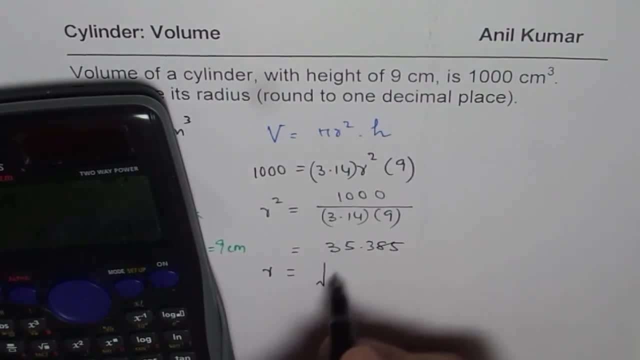 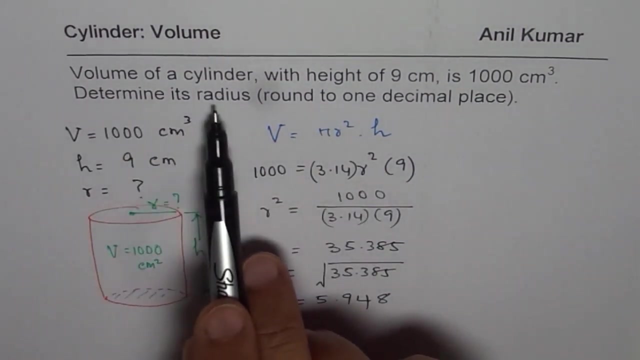 So what should be R? R should be the positive value square root of 35.385.. So let us do square root of our answer. So that is 5.94.. So we can write 9.48 as our radius It says. determine its radius round to one decimal place. 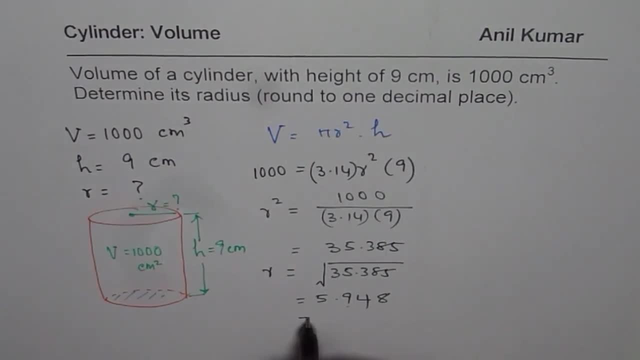 We will round to this. Since 4 is less than 5, we could write this as 5.9 units are centimeters, Right? So I hope this set of calculations is absolutely clear to you. Some of you can actually multiply 9 by 3.14 and then divide 1000 by that number. 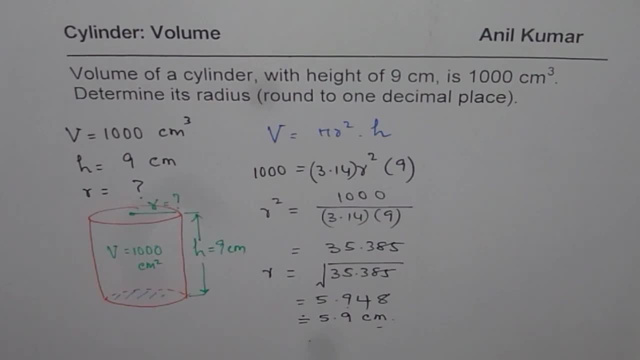 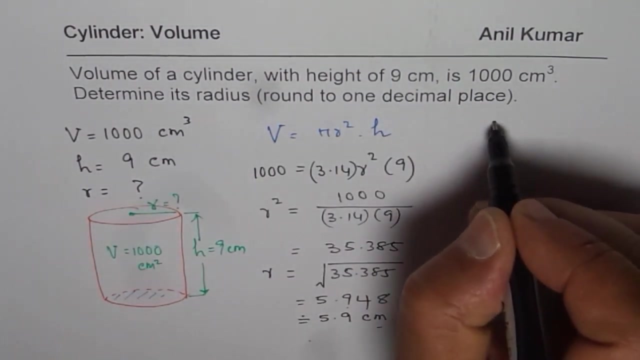 Well, one and the same thing, Anyway. so the idea here is use the formula Volume is pi r square h to find the unknown right. So unknown was radius. You can actually rearrange the formula. also, You can write this as: radius square is equal to volume divided by pi and h. 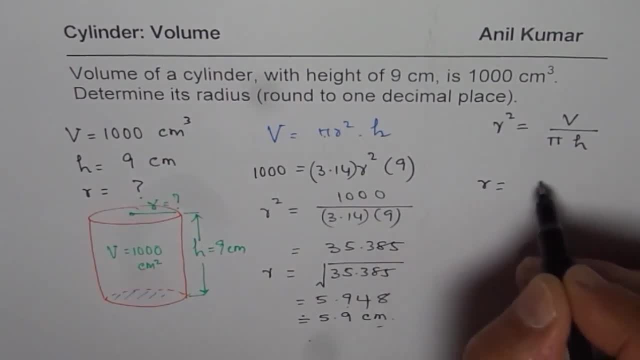 Right Pi and h, And then radius is equal to square root of volume divided by pi and h. Right, So once you do that, you can directly find, So you can say it. So radius equals to volume is 1000 divided by 3.14 times 9.. 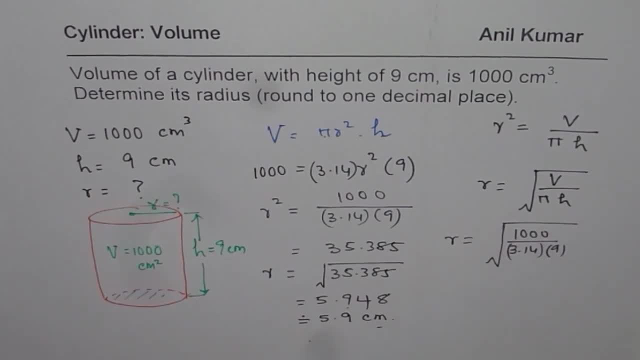 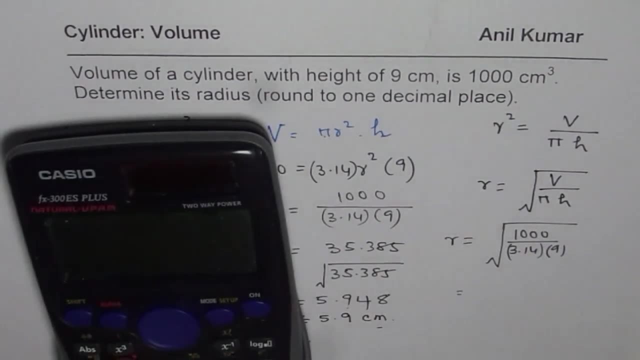 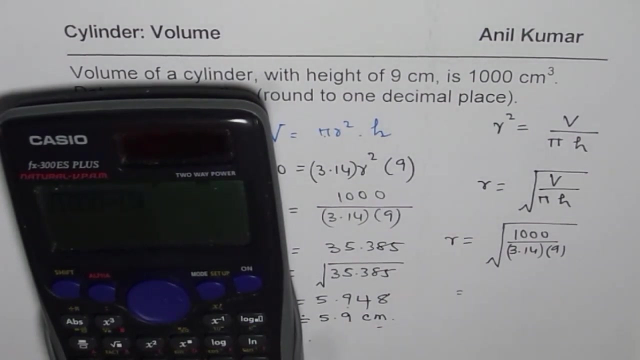 Right, So that is also a way to find radius directly. So you could do that also. That is to say, we have square root of 1000 divided by within brackets, 3.14 times 9, bracket close equal to. So once you do that, you straight away get your answer, which is 5.948, which you can round. 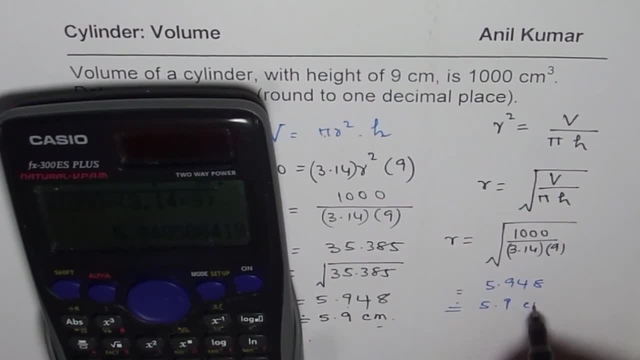 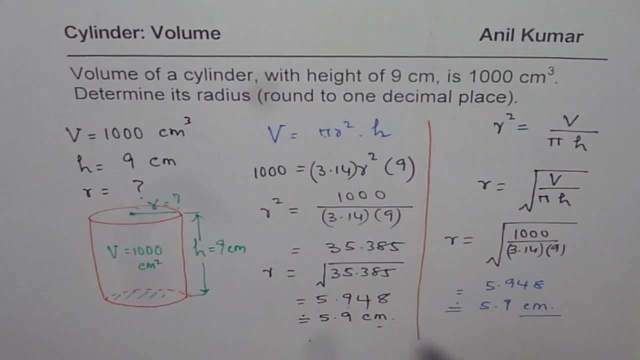 to one decimal place, as 5.9 centimeters. So this is an alternate method And in this method what we have done is we have rearranged the formula in terms of r and then calculated. So you could also apply this method to solve for radius, if volume and height of a cylinder